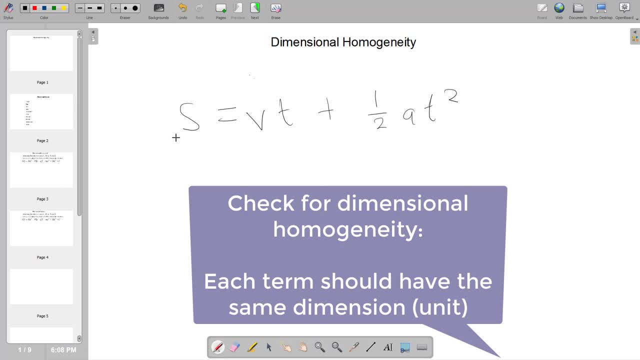 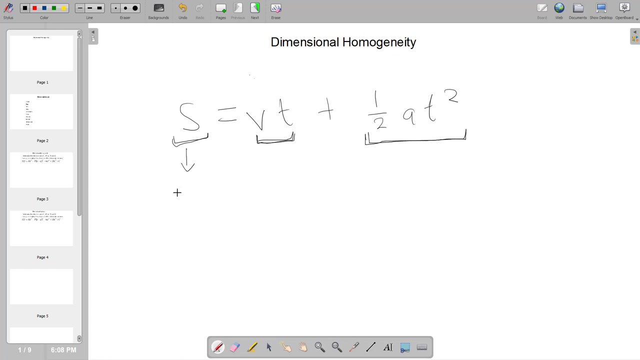 what we are going to check is that every term should have the same units or should have the same dimensions. So the terms are separated by additions. So this whole, this is one term and this is one term. This is a distance. So each unit is meters, This is velocity. 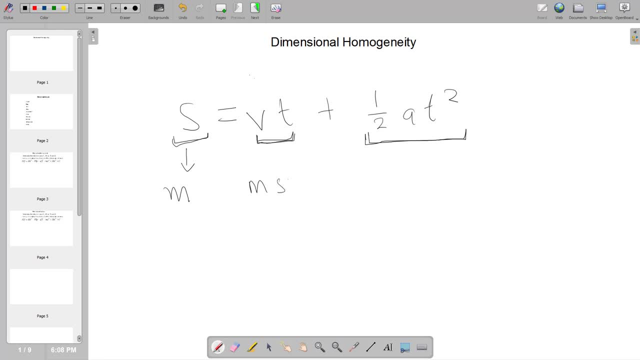 times time. The unit for velocity is meters per second, The unit for time is second per second. So we cancel second. So we have meters, And then here we have half times acceleration, meters per second squared, And then time squared, So second squared, Second squared. 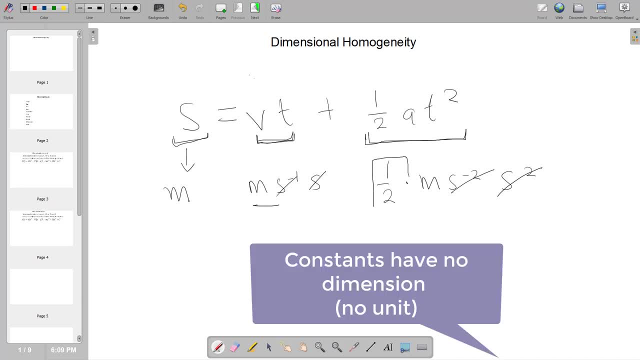 cancels, second squared And constants are dimensionless, So this has no effect on the unit, on the dimension. So again we have meters. So there's meters, there's meters, there's meters. So this equation is dimensionless. 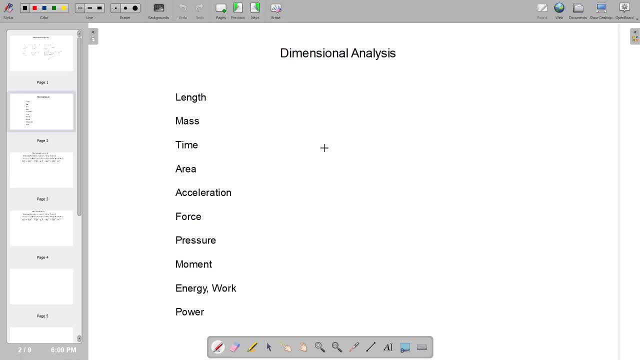 So this is dimensionally homogeneous, Alright. so next up we try to check the dimensions of common quantities. So these are all basic quantities, Length meters. So let's have dimension L, Mass M, And then time, T. Now 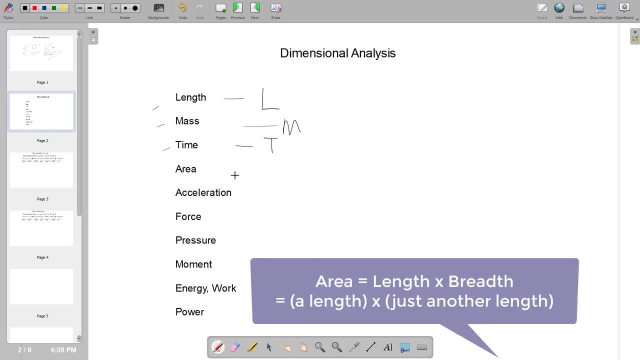 area. Area is sum length, Length, Length times some other length, So it's going to be length times length. So we have L squared for area. So acceleration is a change in velocity over time, So it's some velocity over some time. 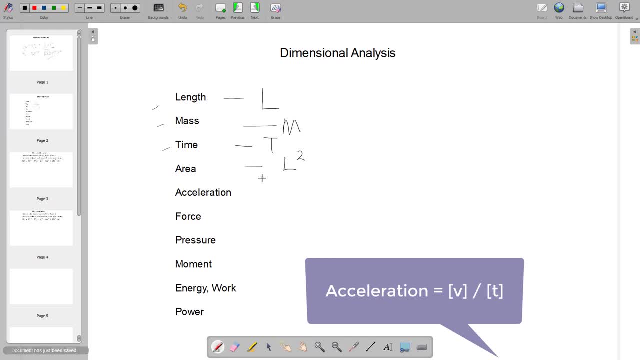 I mean a difference in velocity, which is whose dimension will be a velocity. And then over some time. We know velocity is meters per second, So some distance per some time, So L per T. And then this velocity is changing over some time, So this is over some time, So L per 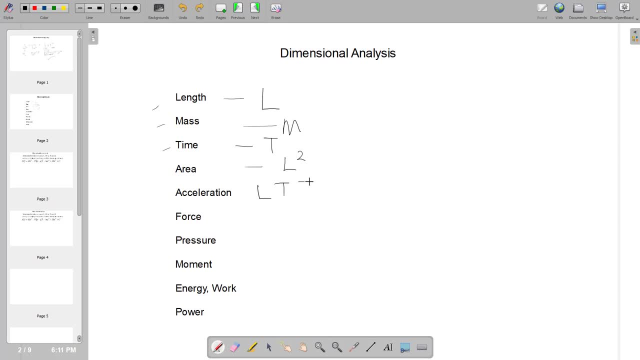 T divided by T then becomes L per T squared, So acceleration has a dimension of L T negative 2.. We know force is some mass times, some acceleration. We know force is some mass times, some acceleration. We know force is some mass times, some acceleration. 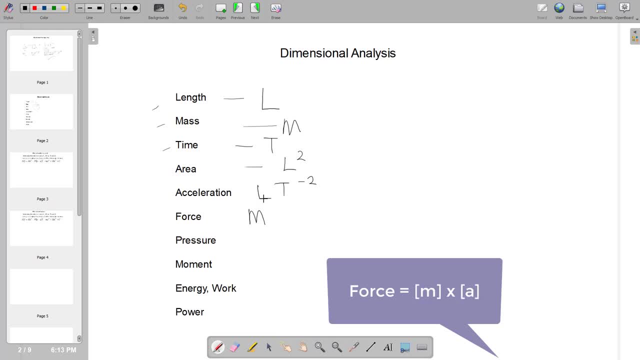 So we have mass multiplying. We already have acceleration here, So we just multiply L T negative 2. Now pressure. We know pressure is some force over some area. So we have force here, M L T or M L per T squared, Dividing some area, and we already have area to be L squared. 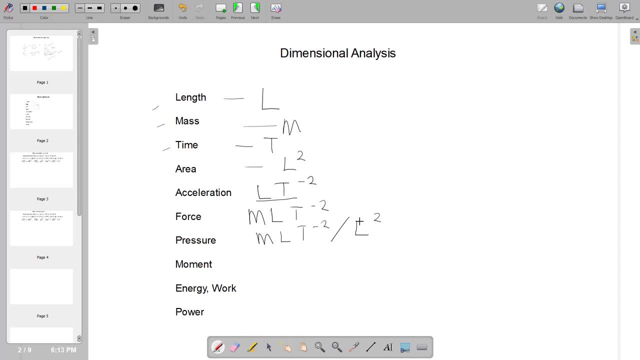 So L squared, Evaluating this, We just have L divided, L squared. We are going to have per L or L to the power negative 1.. So then we have L to the power negative 1. And then for moment, We know moment to be- force, Some force times, some distance. So 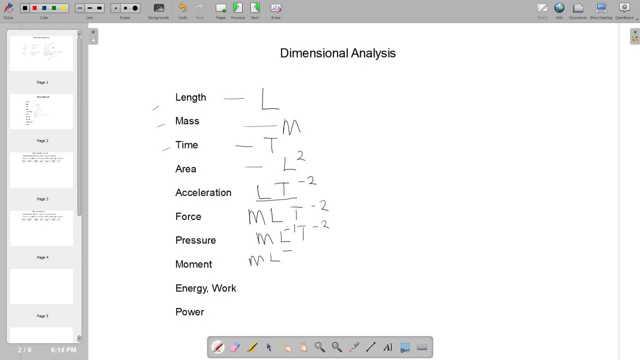 we already have force to be M L, T negative 2. And then we multiply this by some distance, Perpendicular distance, So it still an L. So then we have L multiplying L, So we have M? L squared. Now, energy or work. 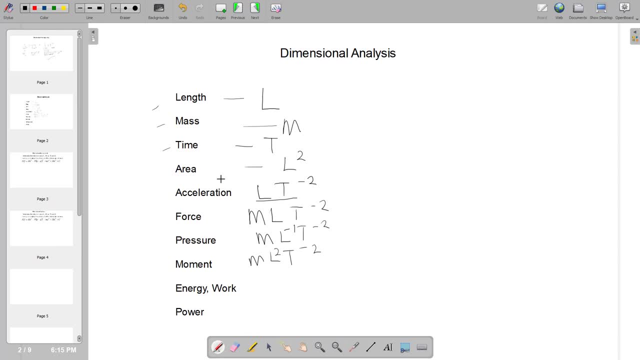 We know: just pick for each of these quantities, Just pick up any formula You know right. And so for energy, we know force times, distance to be energy expanded or work done, So we already have to be MLT. next to then we multiply this by some distance, so again it becomes L. 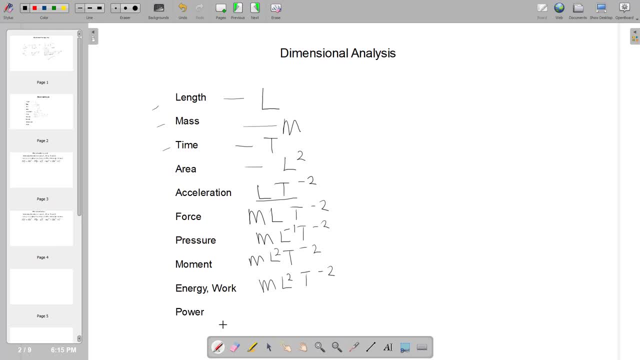 squared, so L squared. and then power will no power to be some, some energy or some work done over some time. so it's this formula, we have here this dimension. we have here ML squared per T squared dividing some time. so we have T to the power negative 2 dividing T to the power: 1. you're going to have T to the power. 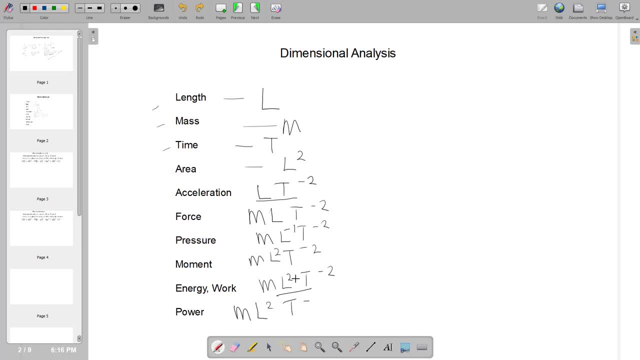 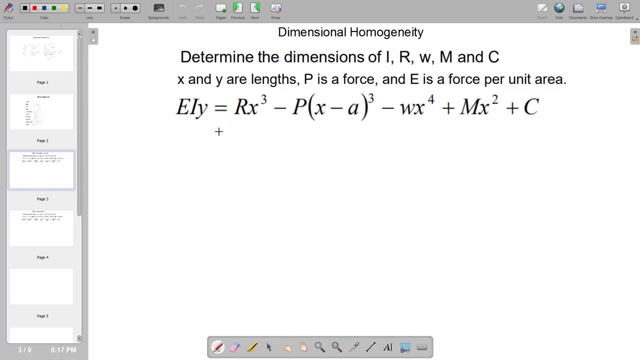 negative 3 over here. so then it's T to the power, negative 3. okay, so we test our understanding with a very interesting question here. so we are to determine the dimensions of I, R, W, M and C in this equation here, and we are told that X and Y are lengths. so they are. 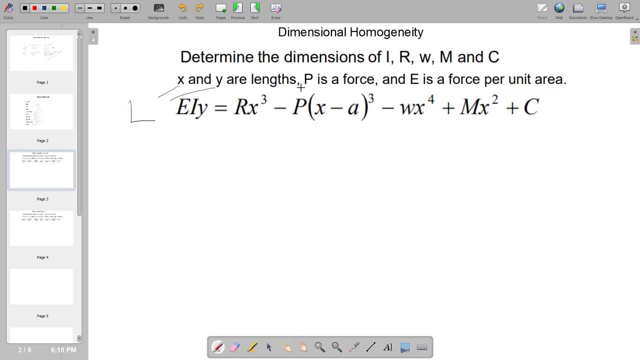 dimensions are just going to be an L, and then we are told P is a force we know. for any force the dimension is MLT or ML per T squared. and then we are told E is a force per unit area. so we expect that the dimension of E is MLT. 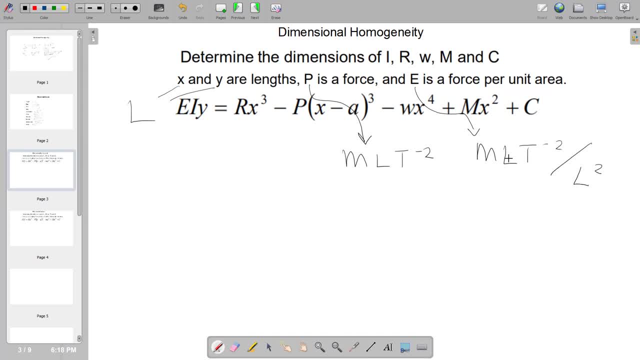 so if we're going to divide the dimension of E by ML T over here, we are going to have a, we are going to have an L squared and we're going to have a force divided by an L squared. where we are going to have an L squared, that's. 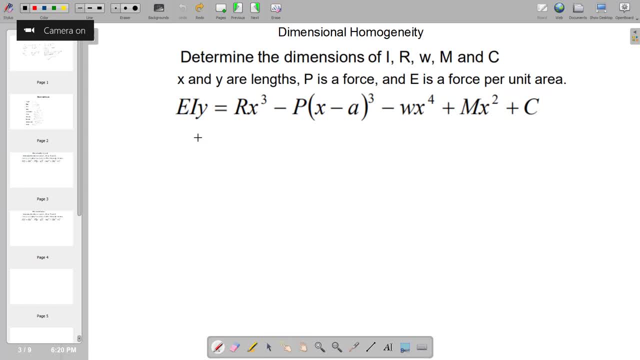 going to be L squared. we're going to have a force divided by L squared, so L divided, L squared. we are going to have an L to the power, negative 1 here. okay, okay. so moving on. how do we approach this now? what do we know about them? 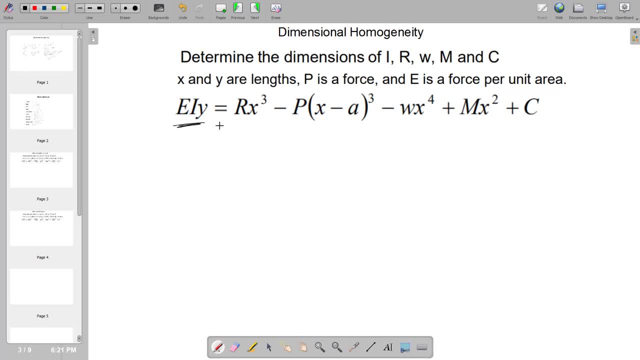 dimensionally homogeneous equations. we know that for each term, or each term in now, look at this- e, i, y will have the same dimension as rx cubed and will have the same dimension as the entirety of p, x minus a or cubed, the same dimension as this, this, and that we also 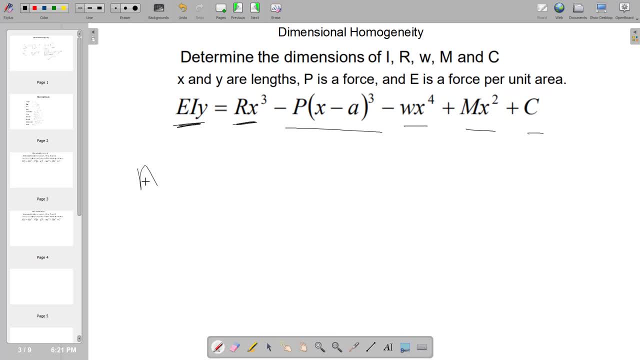 know that you cannot add two quantities that have different dimensions. so if we're having an addition or a subtraction of any two quantities, we are rest assured that these two quantities have the same dimension. so if you look at this particular term, p multiplying the cube of x minus a, 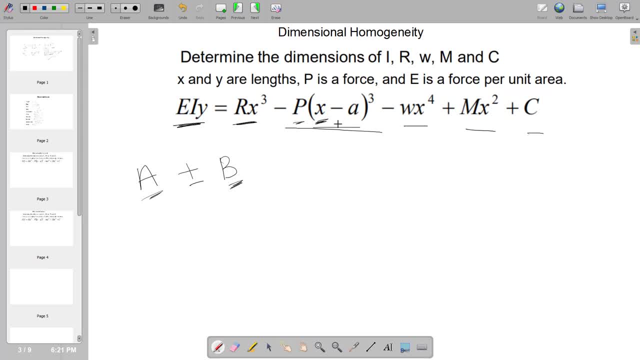 once we are having x being added to or being subtracted from a, x minus a, then we know that x and a have the same dimensions. and if you have any any quantities at all, say some two angles: theta 1 minus theta 2.. if you know theta to be in degrees, then surely theta 2 is in degrees if theta 1 is in radians. 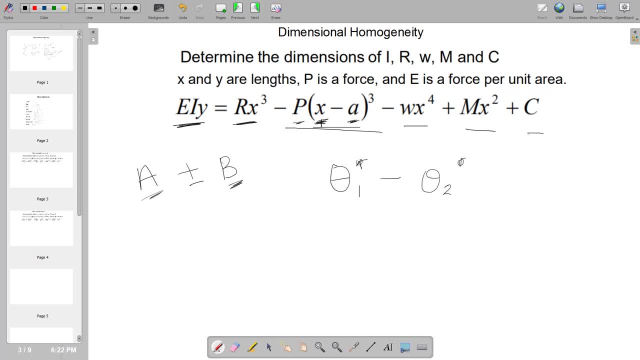 surely theta 2 is also in radians. so we are rest assured that if any two quantities are adding or subtracting, then they have the same dimension. so the question tells us nothing about the quantity a, but the mere fact that a is being subtracted from x, then a has the same dimension. 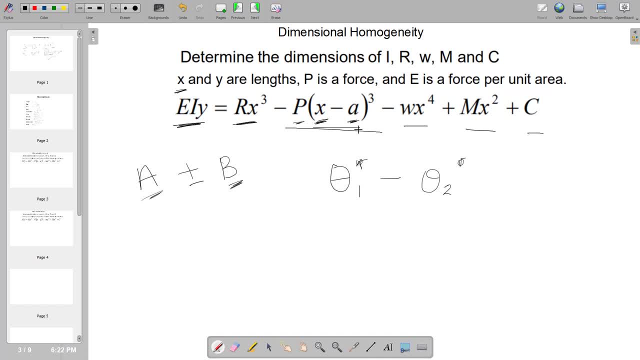 as x, and we are told that x is a length. so definitely a is also a length. so a has a dimension l or a length, all right. so a, say a, has a dimension l. now moving on, we see c sort of alone here, and then rx cube. we know that rx cube is going to have the same dimension. 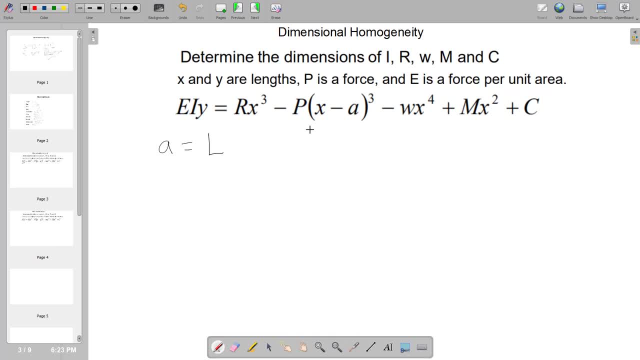 as c. so we can confidently say that c is dimensionally equal to rx cubed. now we know x to be a length, so this is in fact rl cubed. so we know c has the same dimension as rl cubed, but we don't know what r is. this is a force. that's pressure. this is some moment. 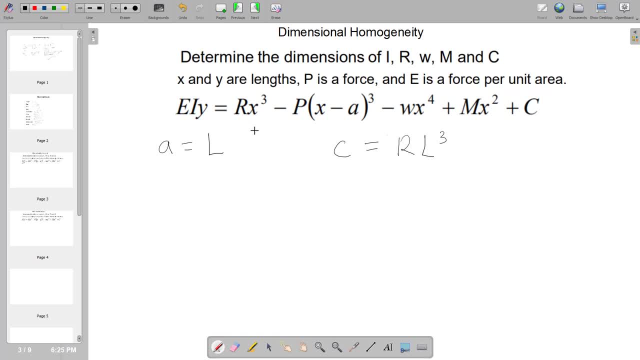 so we are going to have to figure out r out. but you know, we we take, we make use of our knowns to find our unknowns. if you compare rx cubed to pS, quadrupleiqued to p times the cube of x, anyway, we make use of our knowns to find out unknowns. if you compare rx cubed to p, multiplying the cube of x to up and up to x, plus the square of xeb to nah, 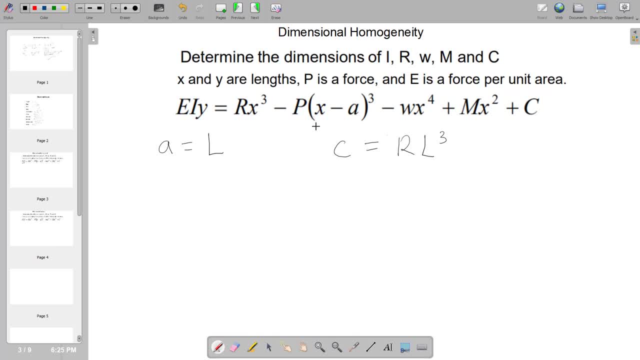 multiplying the cube of x minus a. we already know that x and a are lengths, so both x and a have the dimension l. that means that this entire bracket here has a dimension l, because if you subtract a length from a length, you get a length. so this is actually p multiplying l cubed or a. 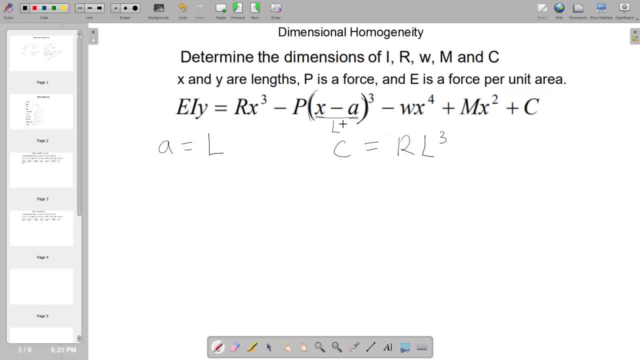 force multiplying an l cubed. so we are going to compare our rx cubed to this force multiplying l cubed. so in fact our rl cubed has the same dimension as our p. we are told in the question that p is a force. so let's just say um, our force has a dimension f, and then this quantity has l as. 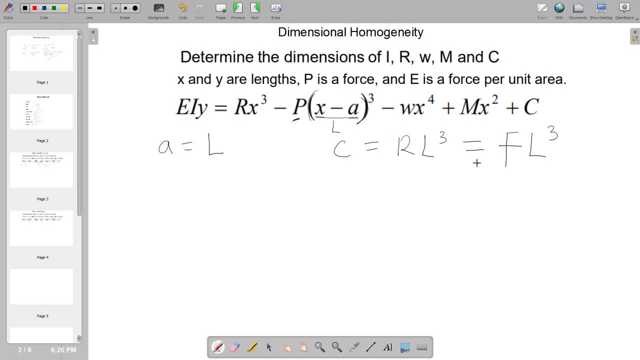 its dimension. so our rl cube is in fact has the same or has the same dimension as fl cubed. so obviously r is equal to l, just by comparing both sides. so our r is in fact a force. now we can say that our c also has the dimension. r is an f, so f? l cubed. 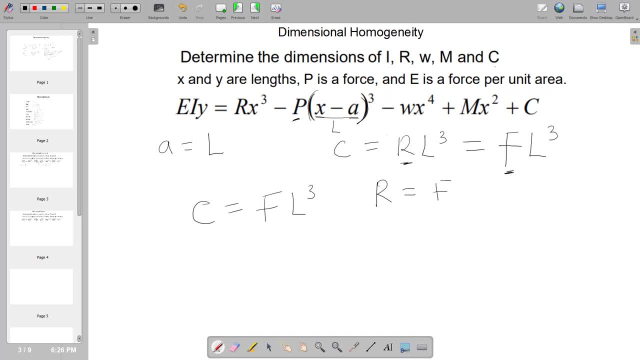 now. so we found c, we found r. now we can compare c to our w, x to the power four. here we know x is an l, x is a length, so our c has the same dimension as this w x 4. x is a length, so l, 4. so, um, we already know our c to be f l cubed. so we say f? l cubed is in. 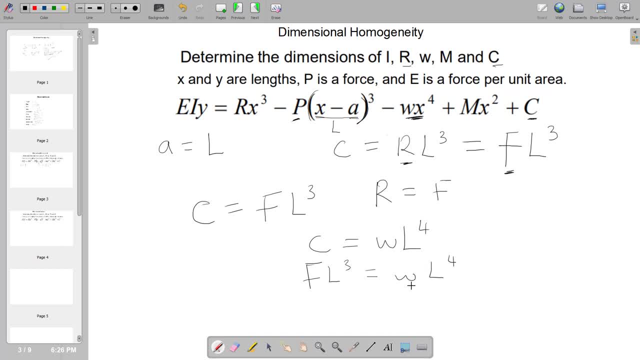 fact equal to w l 4. so we can compare both sides and find out the dimension of w. so we can simply x l 4. x is a length. so if we want to represent the dimension of w, we can say that our w is equal to. 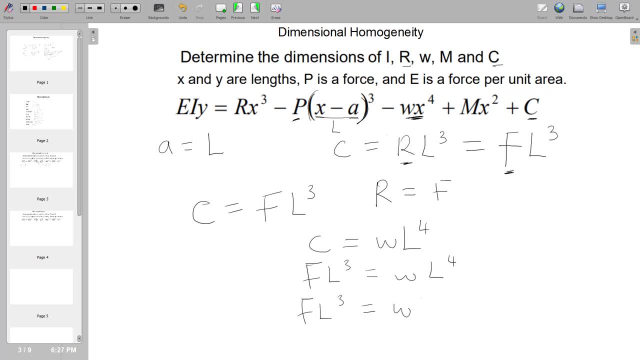 l cubed so we can express our w l 4, because we want it to resemble our left hand side. we can express our um right hand side, as w times l times l cubed. so, as you can see, here we have l cubed, here l cubed. 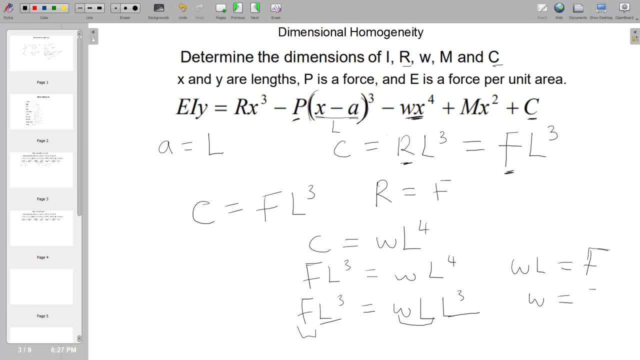 here. so our w? l is in fact a force. so our w? l is a force, force dividing some length, some force, pair, pair, length. okay, so that also gives us our W. we know W. now we need to find M and I. okay, so we have M? L squared here. 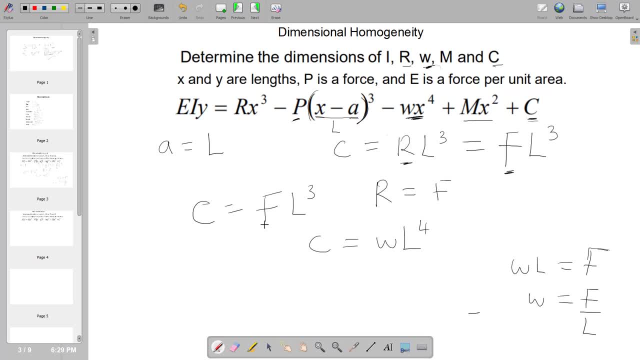 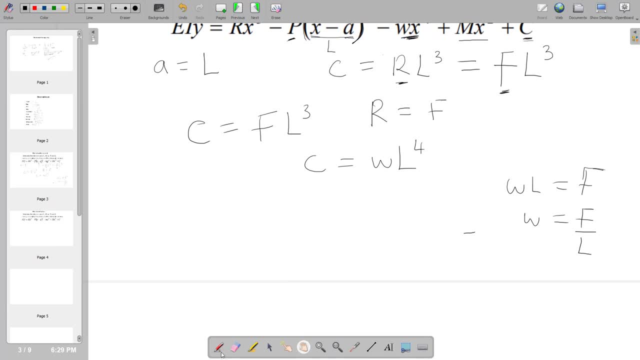 we can simply compare that to our FL cubed. so we say we say our ML squared is a squared. ML squared is simply equal to the dimension of our C, which is FL cubed. so just like we did for W, we can express this, or we can simply just sort of make M the subject. you know, M equals. 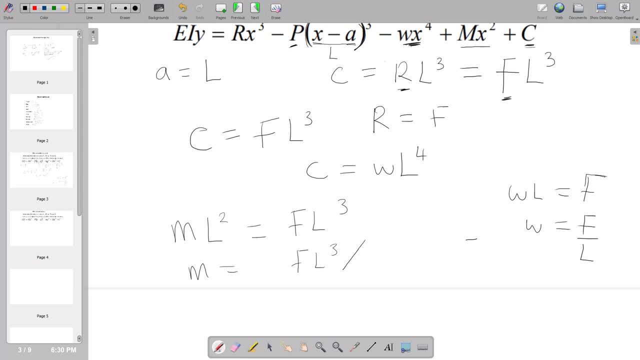 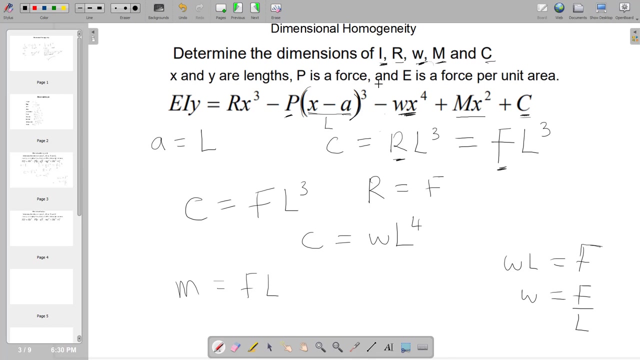 FL cubed L squared. so we divide by L squared, so we just have M to be equal to FL. so M is simply FL. okay, so that gives us our M. now we need to find I, so I'm. where can we find I? we have I in this quantity. 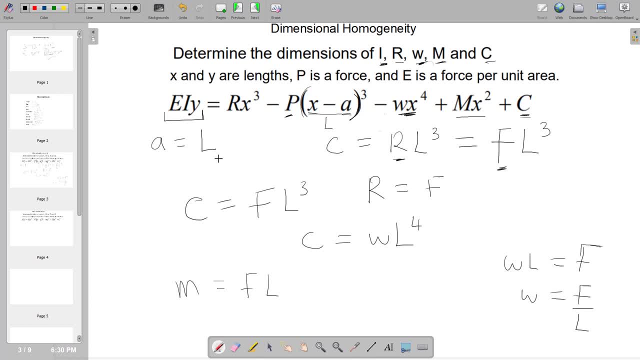 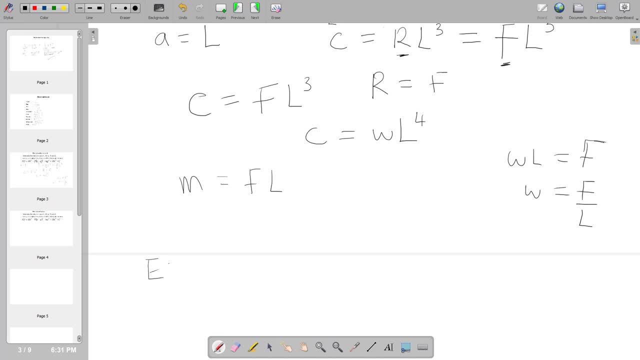 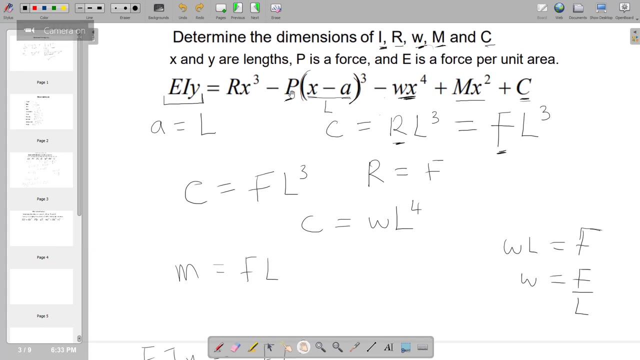 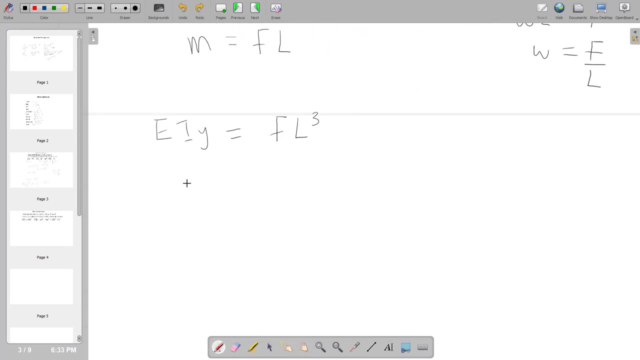 here EIY, so we can compare that to our FL cubed. so for space, EIY, EIY has the same dimension as our FL cube. and in the question we are told that our E is a force per unit area, so it is an F pair L squared, so our E is in fact a force per 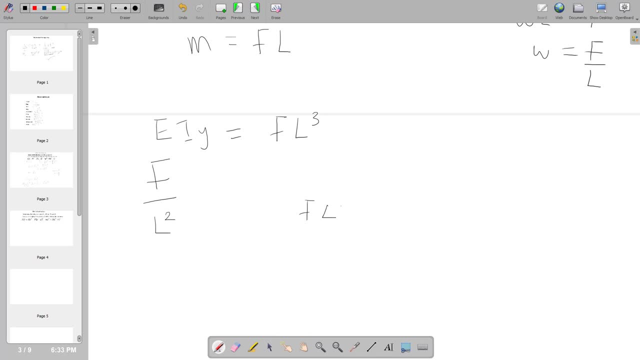 unit area. we can write this as F? L or F pair L squared, so this multiplies our Y. we also told our Y is a length and then our I should have the same dimension as FL cubed. so we just simplify: L cancels this, so we have F I pair L should be F L cubed. then this is: 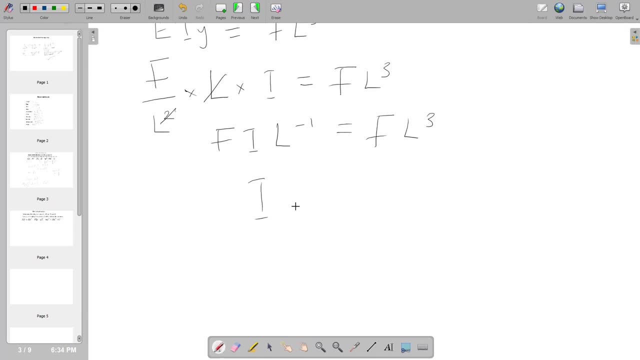 just a matter of simplification. so our I should be equal to F L cubed. our F moves to this side, so we have a pair F, and our pair L moves to this side, so we have an L. so our pair F cancels our F. our L cubed just multiplies L, so we have 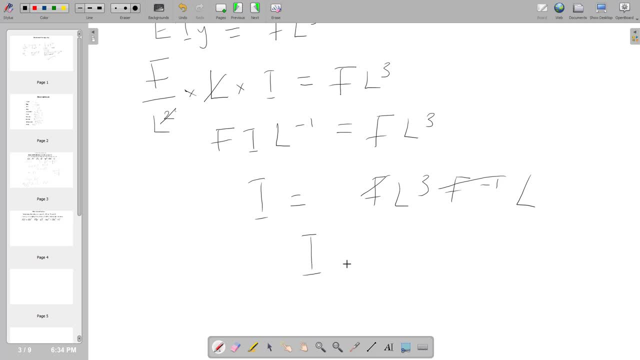 L to the power 4, so our I is equal to L to the power 4. right, there are many approaches to simplifying this. so we have a pair: L to the power 4. so we have bunch of sides. so our I, if we add this, I can 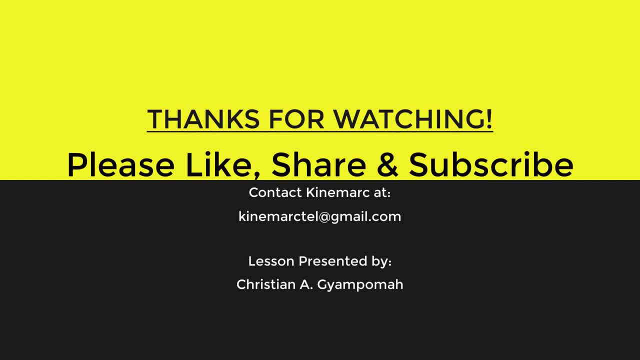 find L to the power 4 and the logo L if I plot any of these on my table, so I